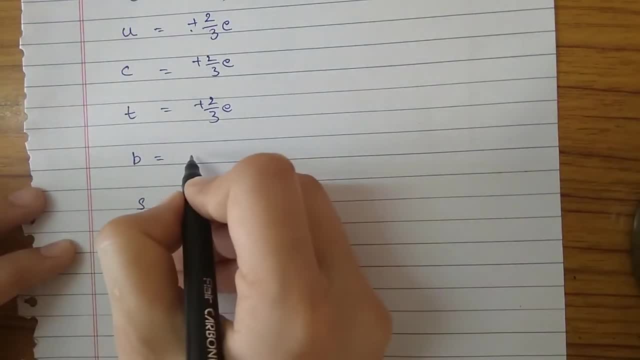 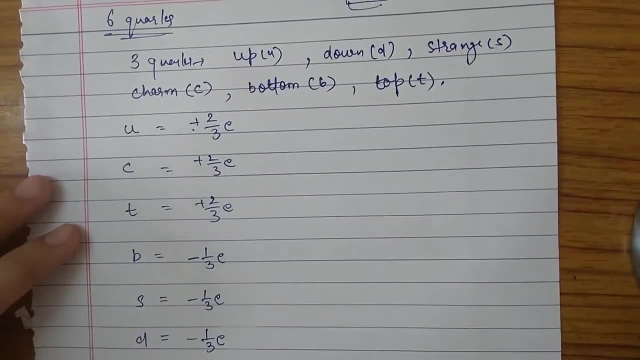 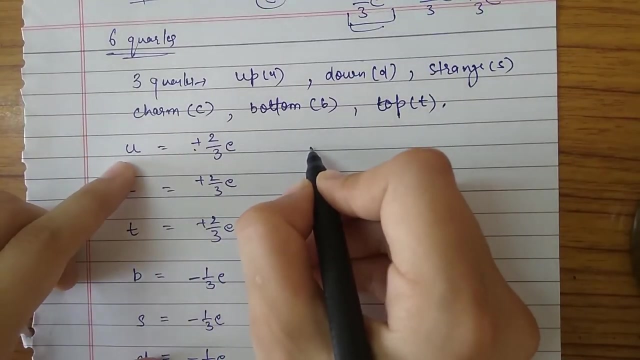 quark and down quark. they have charges of 1 by 3 E minus 1 by 3 E And the anti quarks of these quarks have opposite charge, that is, the anti quark of up quark is denoted by U bar. 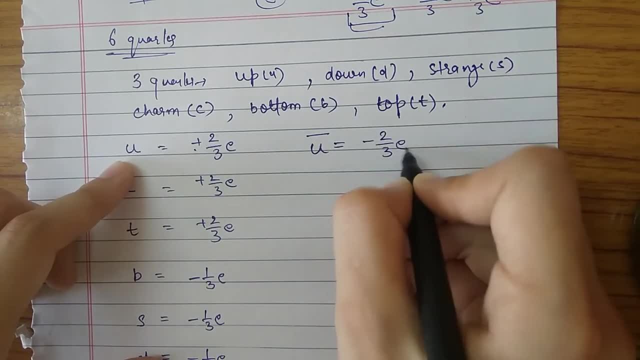 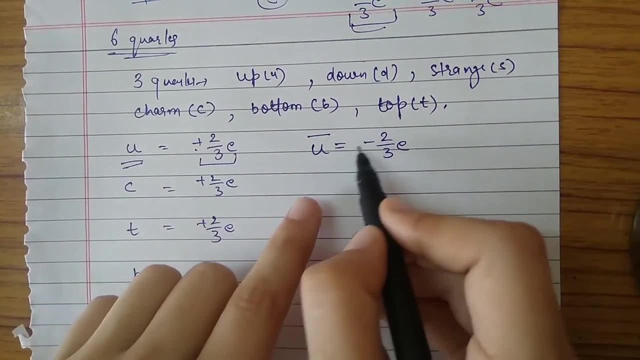 And its charge is minus 2 by 3E. The up quark has charge plus 2 by 3E and this anti quark has the opposite sign of the charge, So it will have minus 2 by 3E. Similarly anti quark. of charm quark will be, will have opposite charge. So So if a quark is positive, then the quarto is positive, so it will have 2 by 3.. Similarly, anti quark of charm quark will have positive charge. that is U bar, which means U bar. So the 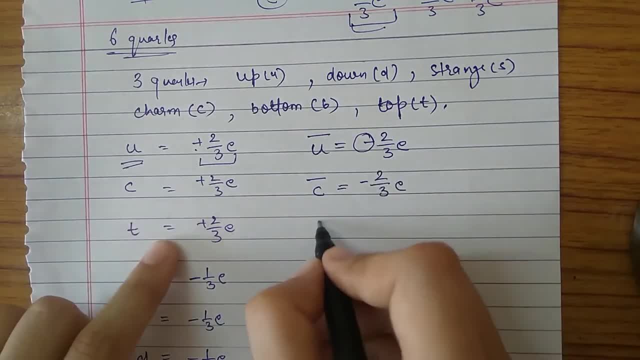 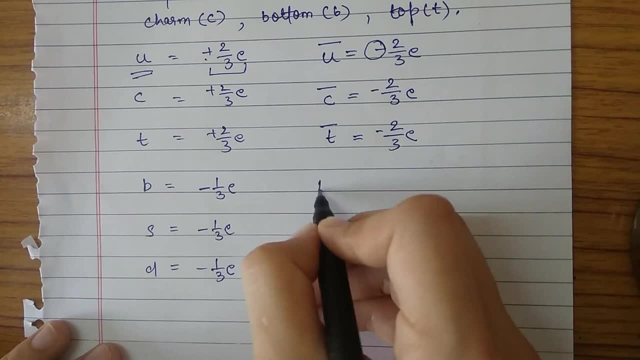 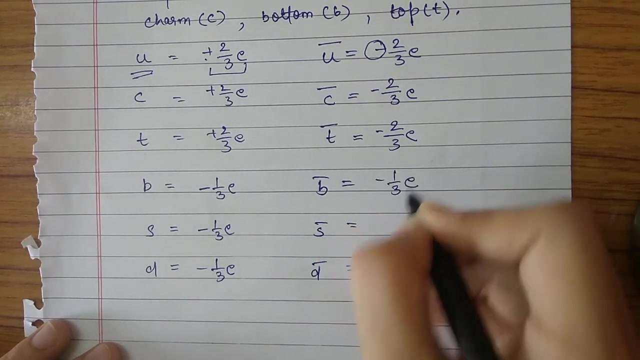 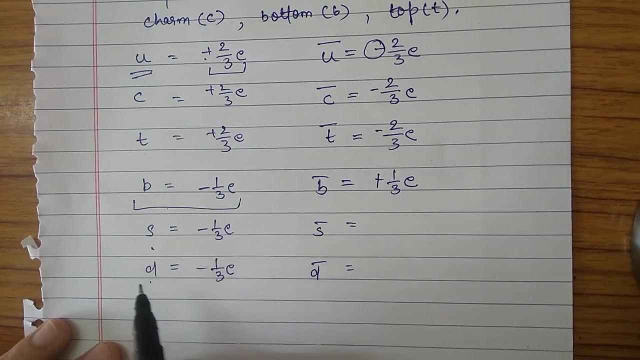 will have a minus 2 by 3e charge. anti quark of top quark will have minus 2 by 3e charge. similarly the anti quark of bottom, strange and down quark. they all will have charge of plus 1 by 3e. the quarks, bottom quark, strange quark and down quark, have minus 1 by 3e charge. 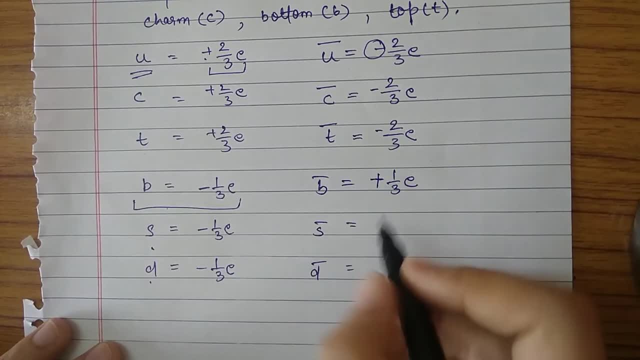 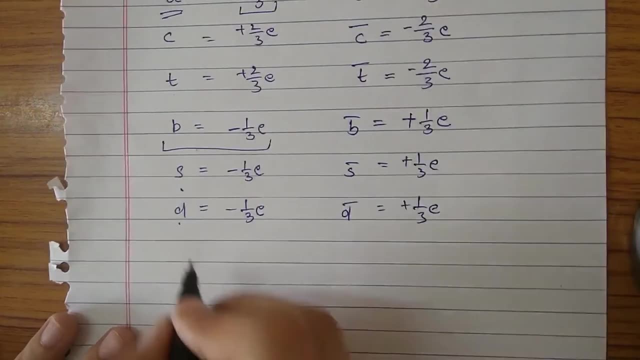 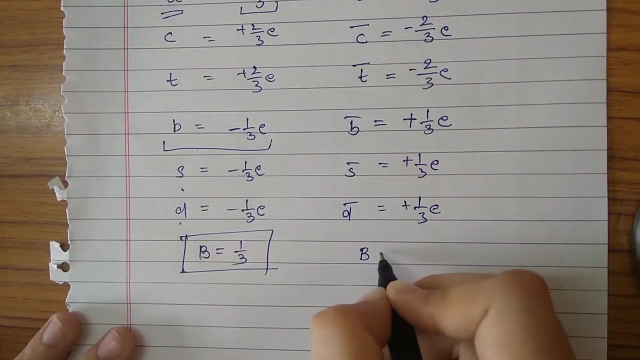 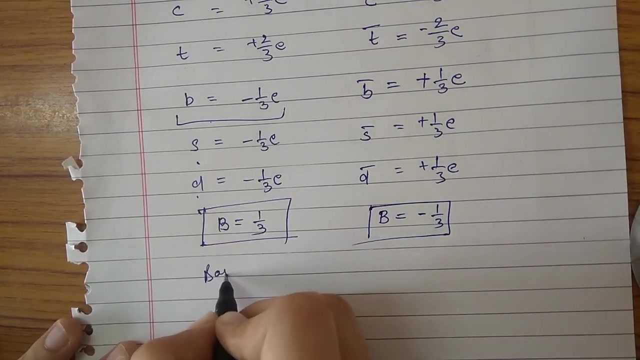 and the anti quark will have opposite charge, that is, plus 1 by 3e. now each quark has baryon number b equal to 1 by 3. this is for the quark, and each anti quark has baryon number minus 1 by 3 and since each baryon, each baryon is made up of three quarks. 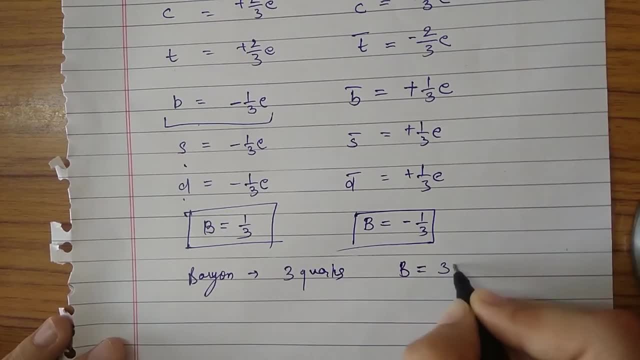 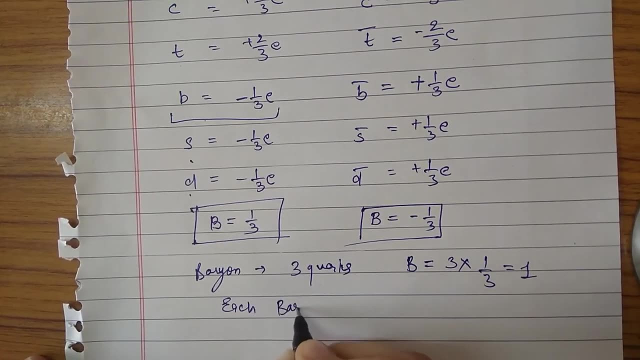 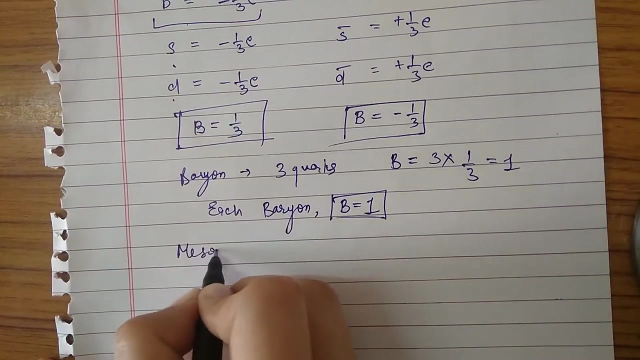 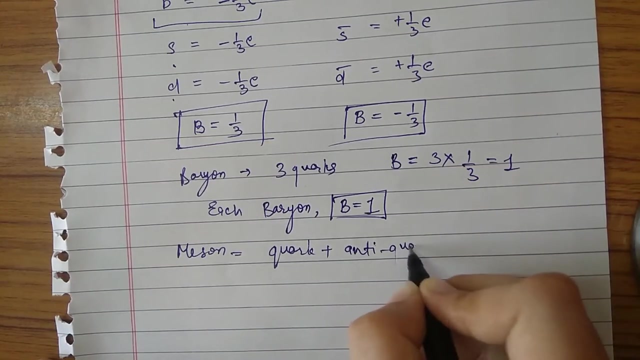 so baryon number of a baryon will be equal to three, into baryon number, that is one. so each baryon will have baryon number equal to one. now a meson. a meson is made up of one quark and one anti quark, so the baryon number of meson will be b equal to 1. 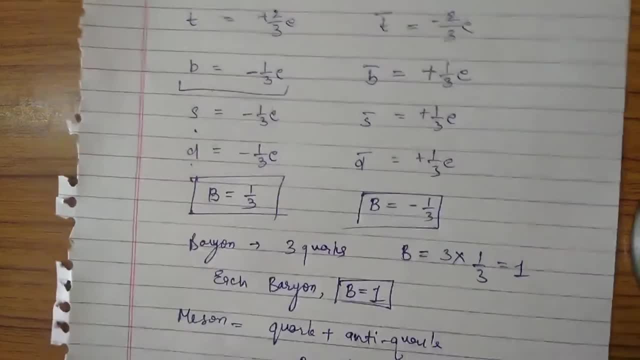 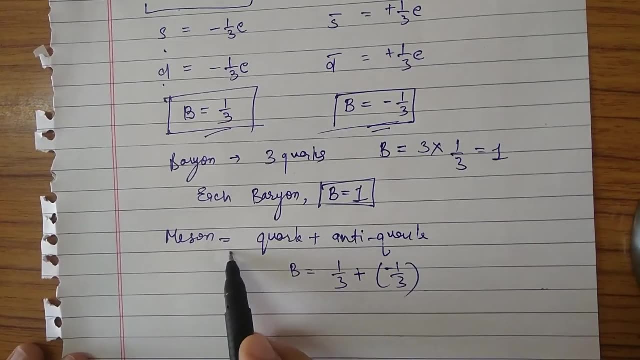 by 3 plus minus 1 by 3, since baryon number of an anti quark is minus 1 by 3 and baryon number of a quark is 1 by 3. so, meson for meson, baryon number will be 1 by 3 plus minus 1 by 3. this will be. 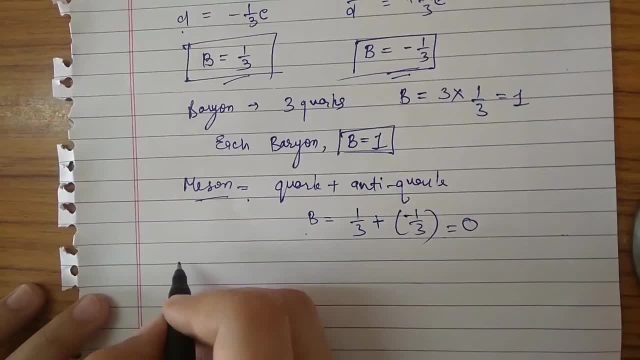 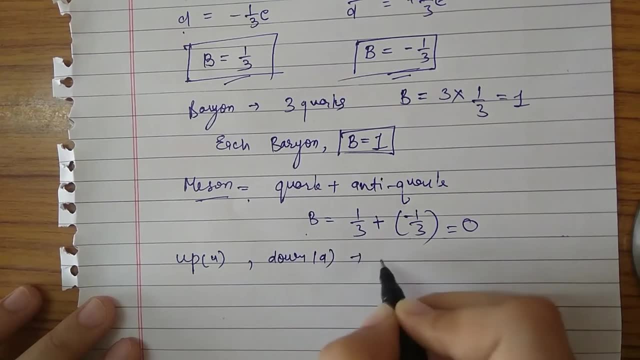 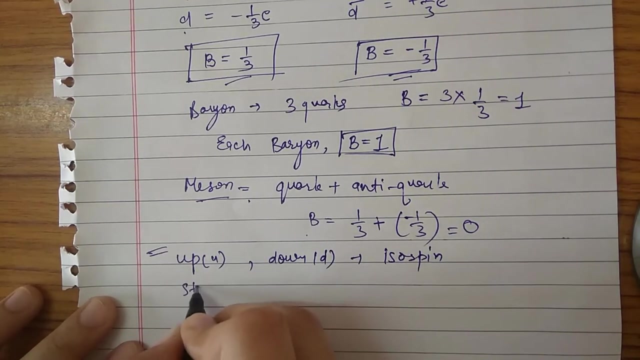 equal to 0. now only two quarks, that is up quark and down quark. they have isospin. only up quark and down quark. they have isospin. Only up quark and down quark have isospin and strange quark. 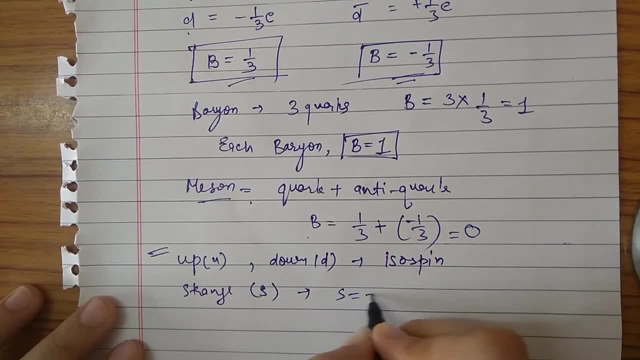 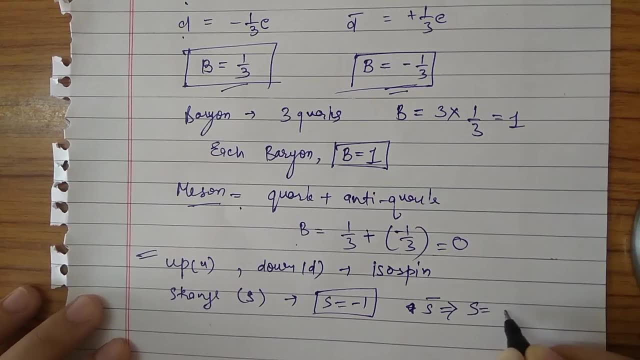 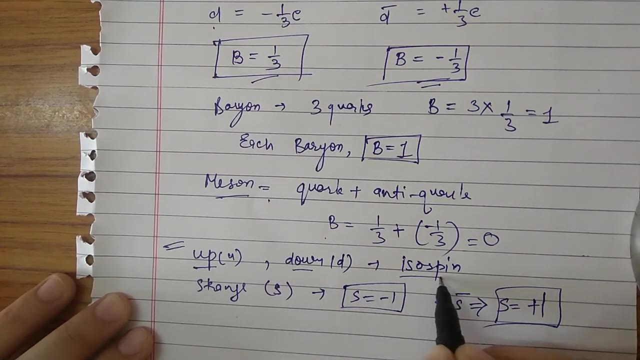 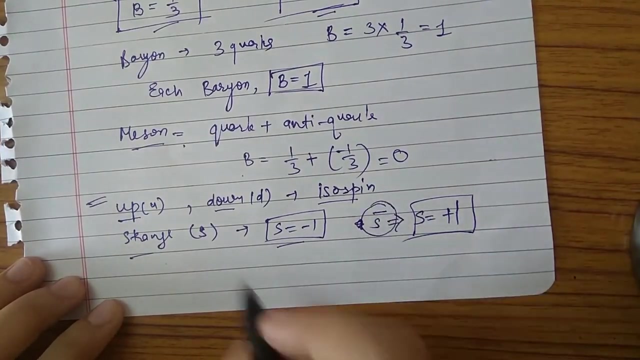 has strangeness s equal to minus 1, and its anti-quark s bar has strangeness equal to plus 1.. So up quark and down quark have isospin. strange quark has strangeness s equal to minus 1, and the anti-quark of strange quark has strangeness equal to plus 1 and. 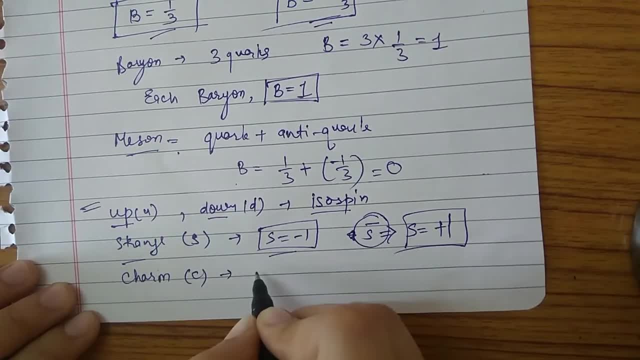 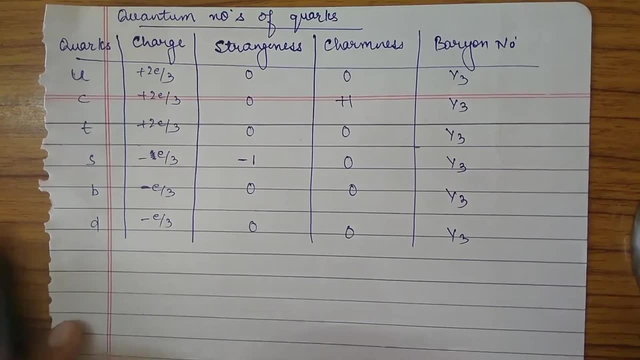 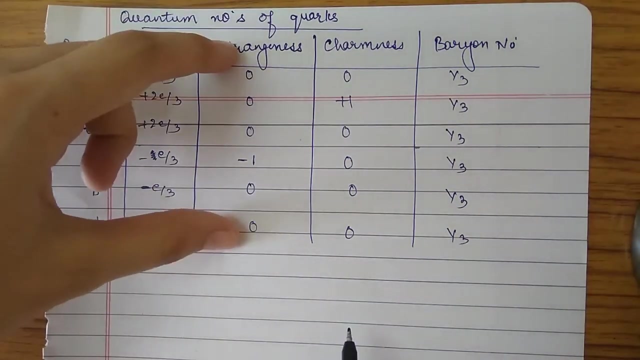 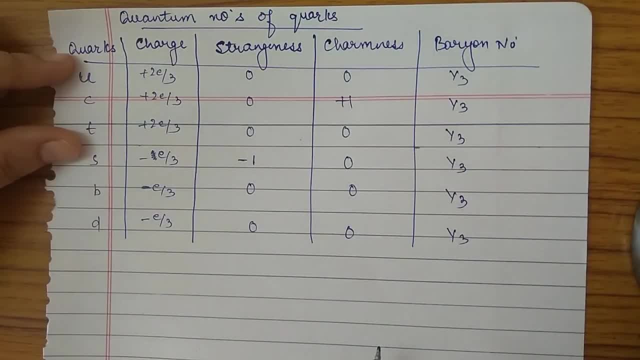 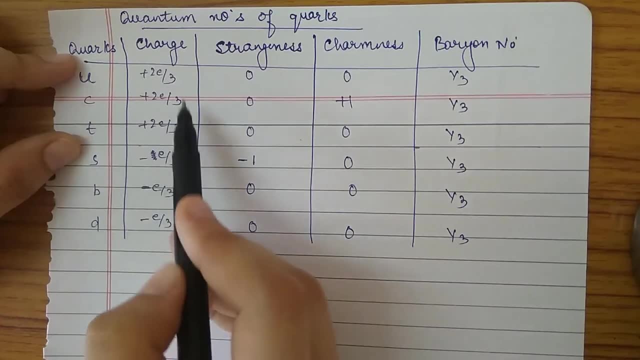 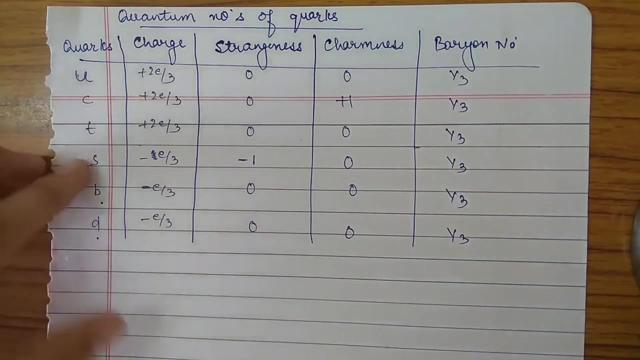 charmness and baryon number. Now, as I have earlier told you that, up, quark, charm, top, they all have charges plus 2 e by 3. Strange bottom and down quark has charges minus e by 3. Now, only strange quark has strangeness equal to minus 1. Others will have zero. 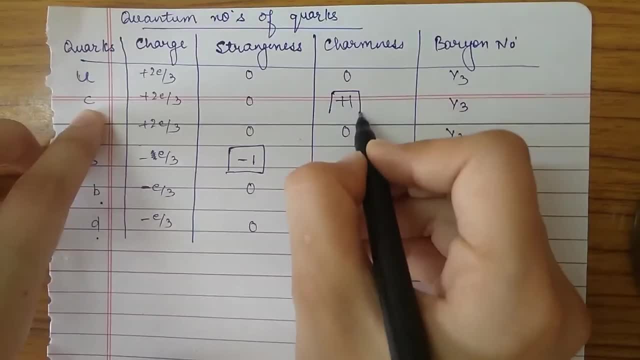 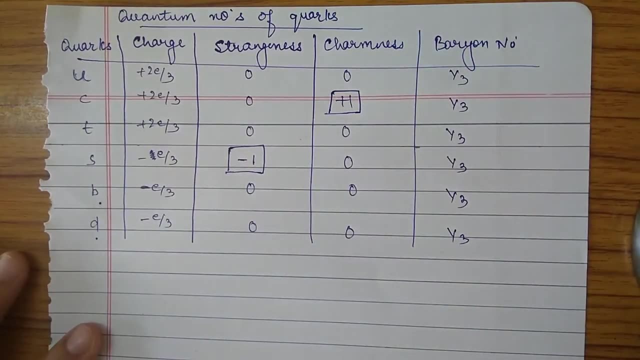 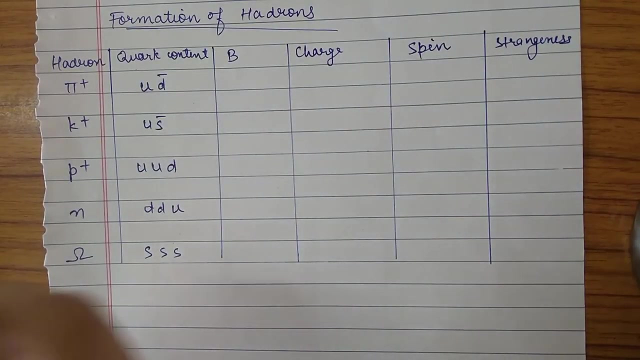 strangeness. Charm quark has charmness equal to plus 1.. Others will have zero charmness and baryon number for every quark is 1 by 3.. Now we will see the formation of hadrons. For this we need the quarks u b, s? u bar, b bar and s bar. So first we will see the 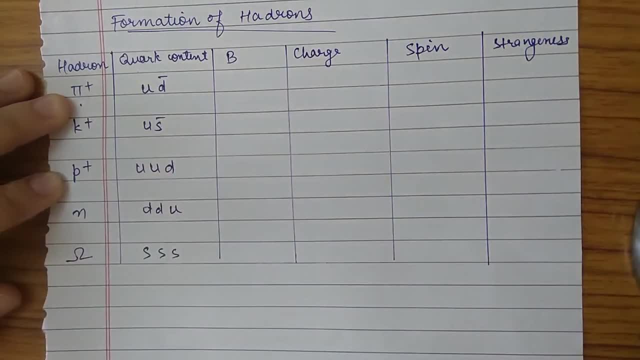 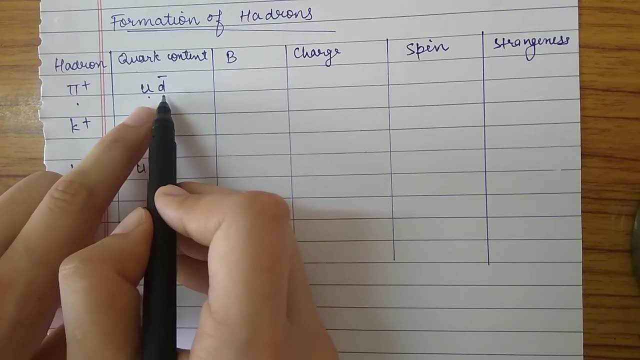 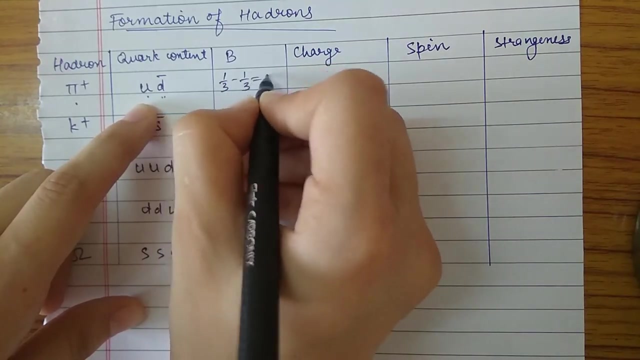 pi positive hadron. For this we need one quark u and the anti-quark of down quark, that is, d bar. Now for this baryon number will be 1 by 3 minus 1 by 3, equal to 0.. 1 by 3 for. 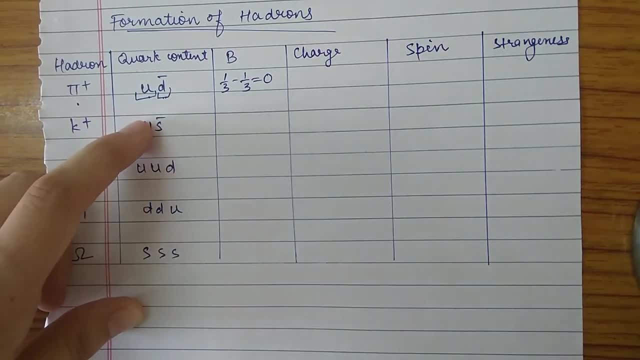 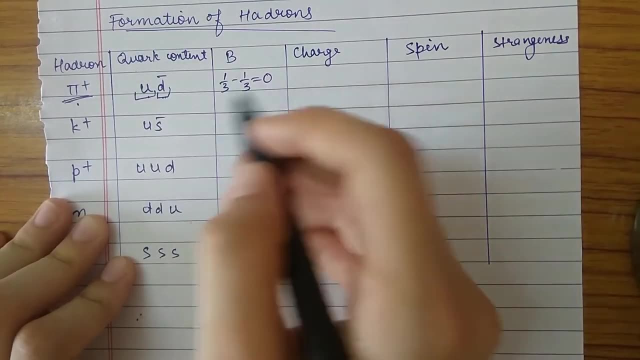 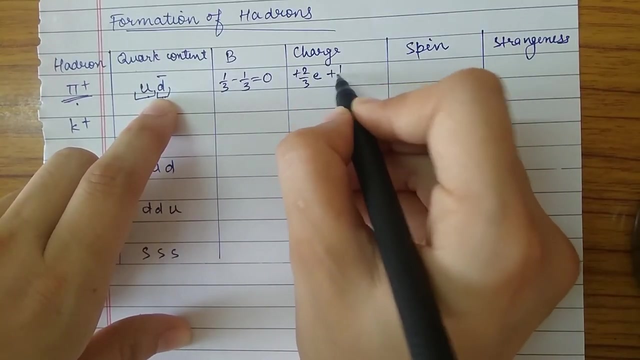 up quark and for this anti-down quark we have baryon number minus 1 by 3.. So the baryon number of pi plus will be equal to 0.. Now charge will be: charge for u is plus 2 by 3 e and for d bar it will be plus 1 by. 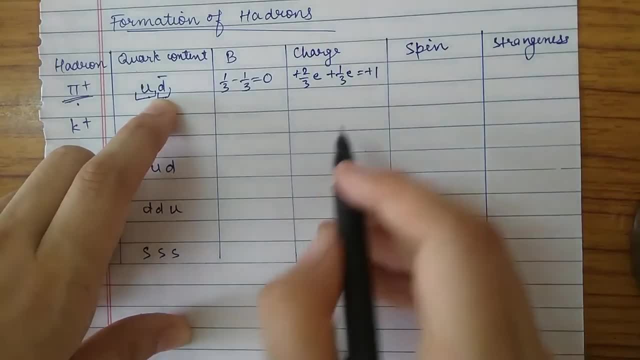 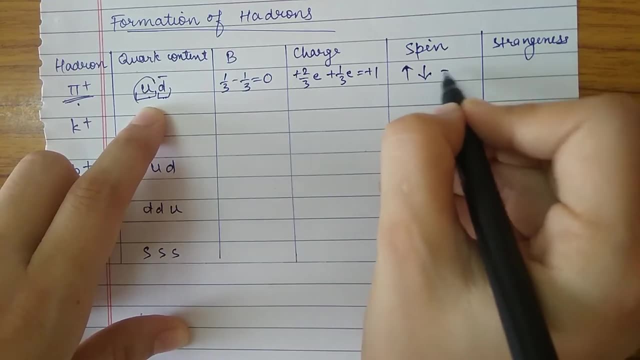 3 e, which will be equal to plus 1.. Now spin of up quark will be up spin and for the anti-quark it will be downward, So the total spin will be equal to 0. and strangeness since there. 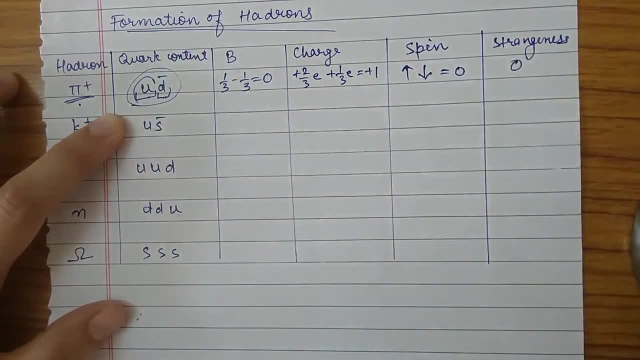 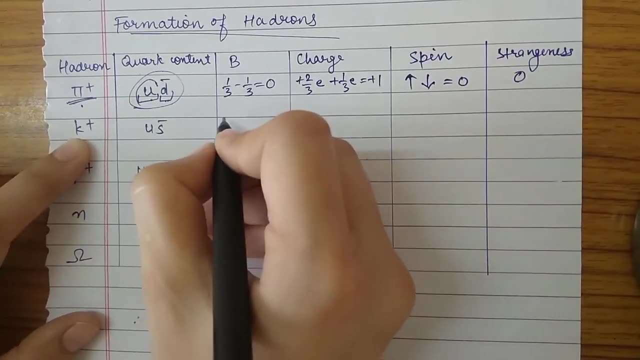 is no strange quark in this, so strangeness will be equal to 0.. Similarly for k k bar baryon, positive K plus hadron, we have baryon number 1 by 3 for up quark and minus 1 by 3 for. 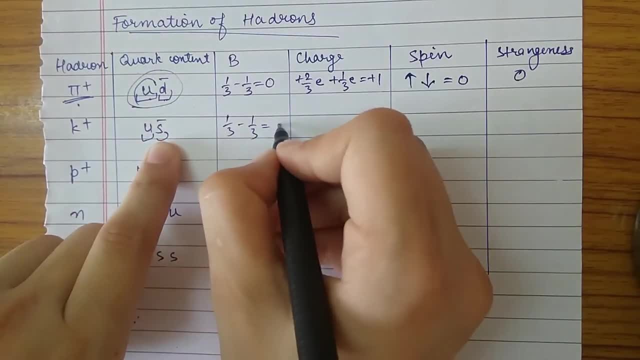 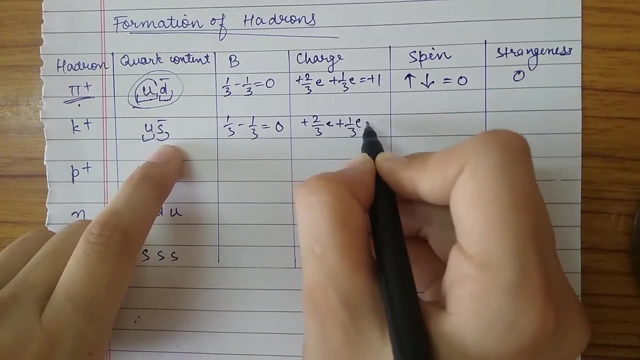 anti-quark, anti-quark or strange quark. So it will be equal to 0 and the charge will be plus 2 by 3 E and plus 1 by 3 E, which will be equal to 1, and its spin will again equal to 0.. 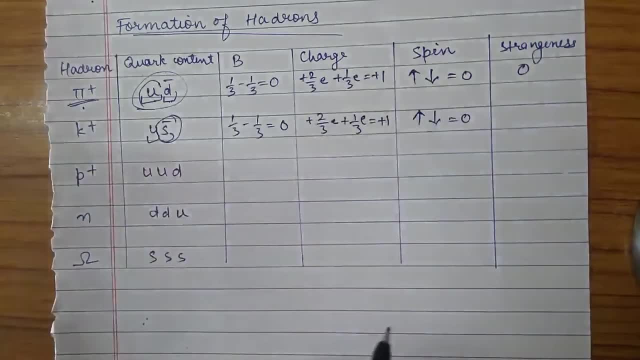 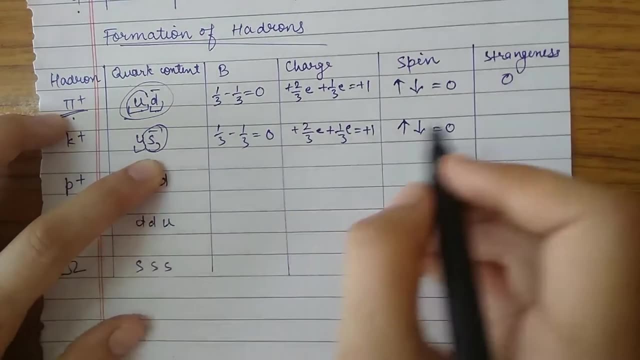 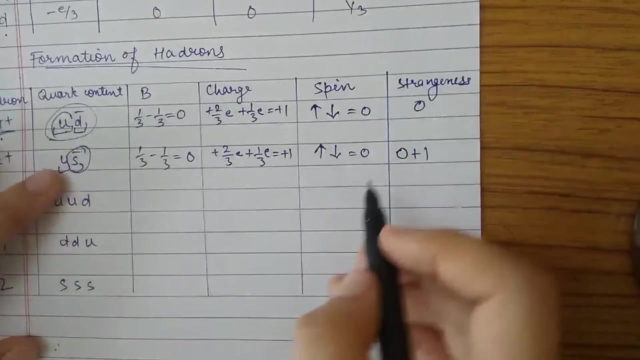 So, since there is one strange anti-quark or strange quark, and we know that strangeness of anti-quark, anti-quark or strange quark is equal to plus 1.. So the strangeness will be equal to 0 for up quark and plus 1 for this S bar, it will be equal to plus 1.. Now in this we have two up. 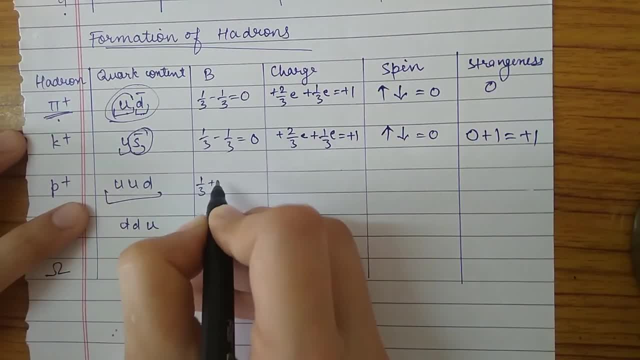 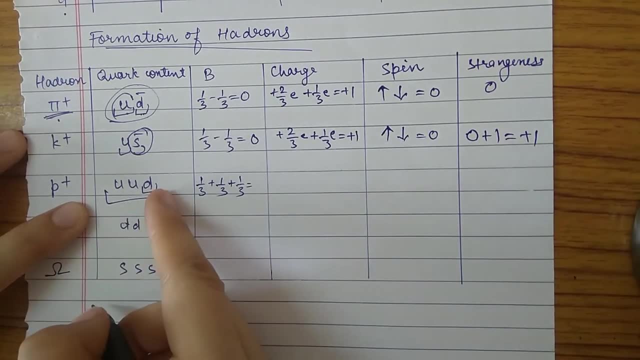 quarks. So the baryon number will be equal to 1 by 3 plus 1 by 3. and since there is one strange anti-quark or strange quark- and we know that strangeness of anti-quark, Since it is a down quark, so the baryon number will be 1 by 3 for this also, and total baryon number will be equal to plus 1.. 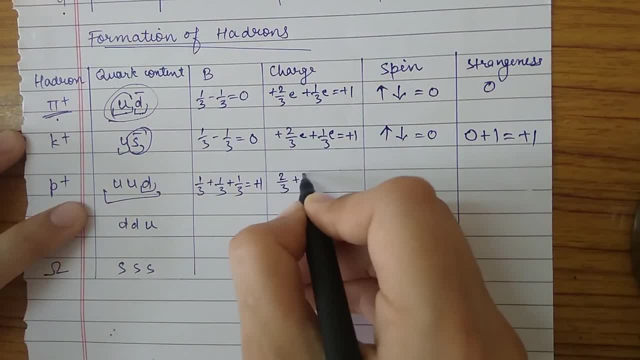 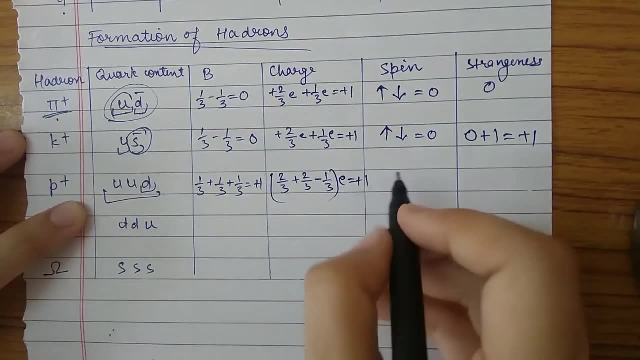 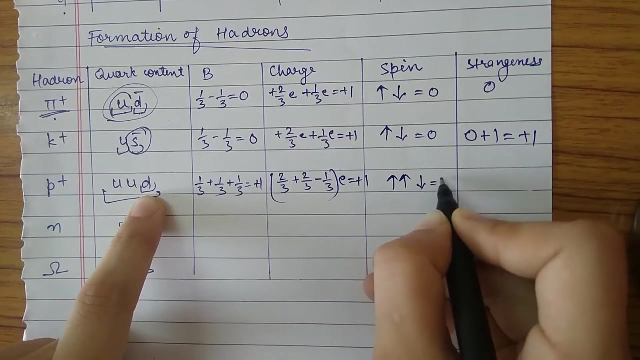 And charge will be equal to plus 2 by 3. plus 2 by 3 and minus 1 by 3 e equal to plus 1.. And spin will be equal to: for up quark: the spin is up and for down quark, spin is down. so it will be equal to 1 by 2.. 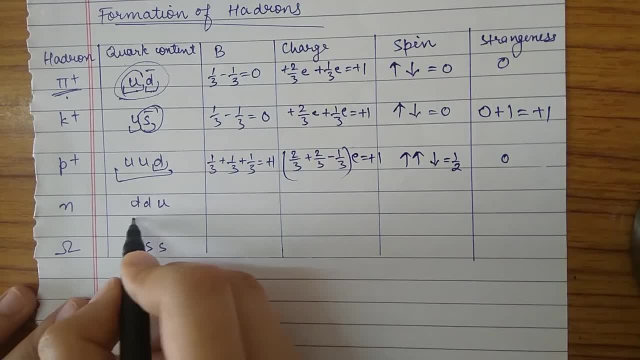 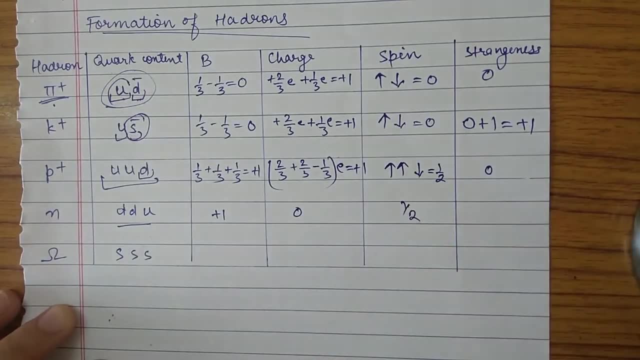 And strangeness will be equal to 0.. Now for this we have baryon number equal to plus 1 and charge will be equal to 0, and spin will be equal to 1 by 2 and the strangeness will be equal to 0. 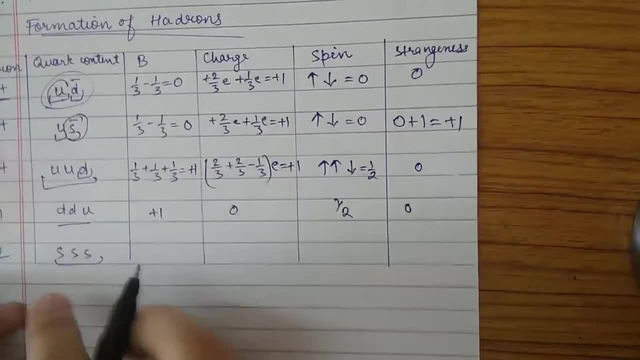 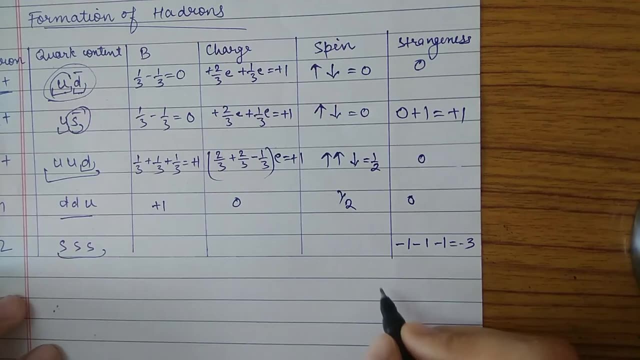 For this, since there are 3 strange quarks, so we will have strangeness equal to minus 1 minus 1. minus 1 equal to minus 3, because strangeness for strange quark s is equal to minus 1.. Now baryon: number of strangeness. 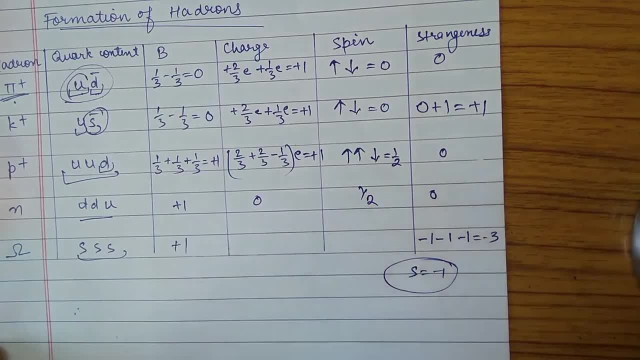 So we have strange three strange quarks will be equal to plus 1.. Charge will be equal to minus 1 by 3, minus 1 by 3 minus 1 by 3 e equal to minus 1.. So spin is up. spin for all these strange quarks. 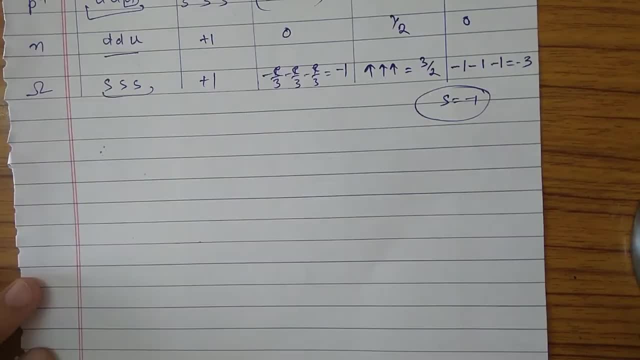 The total spin will be equal to 3 by 2.. Now a problem arose for same particle having spin 1 by 2. That upperspin problem was that it may have two or three quarks of same nature. Now to avoid violation of Pauli's 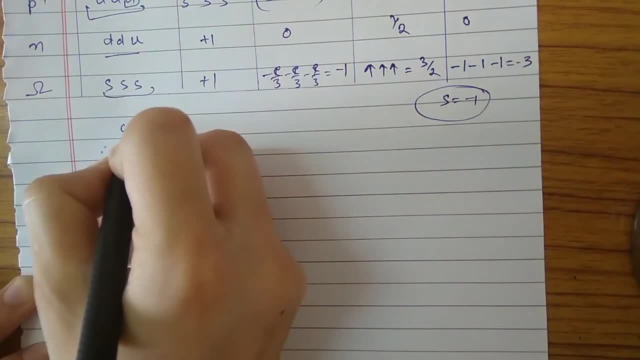 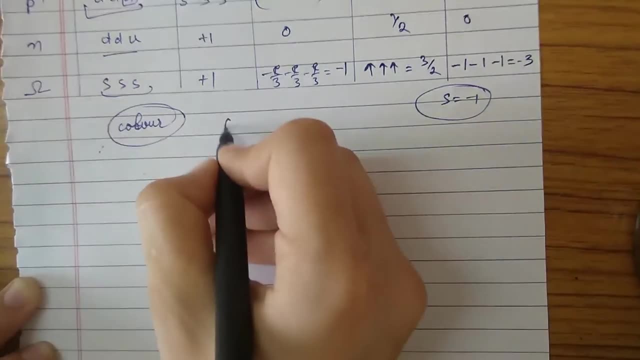 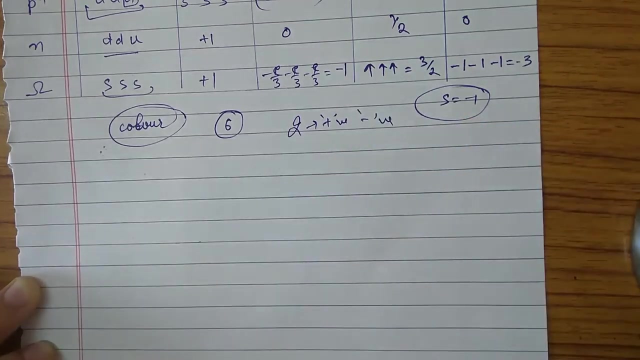 exclusion principle. an additional property of color was introduced. It was said that the quarks and anti-quarks have six different ways rather than two ways. two ways of plus charge or negative charge. So there came six different ways of identifying the of explaining the quarks. 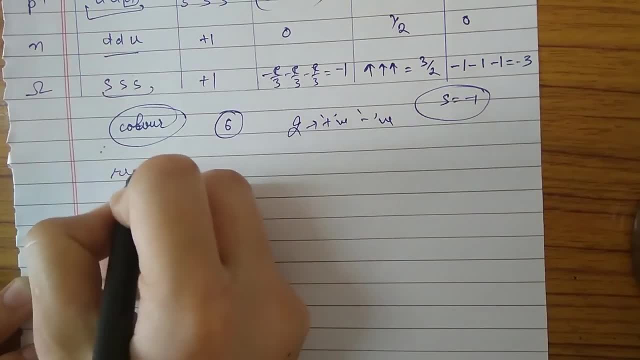 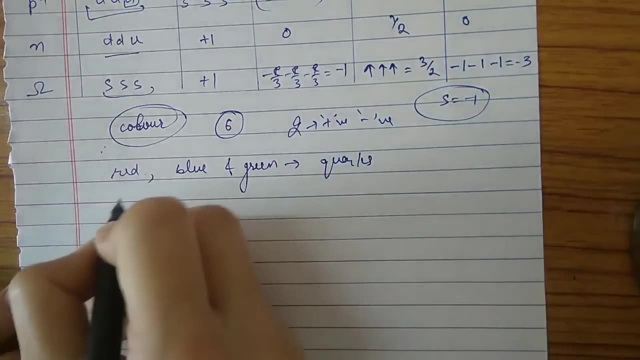 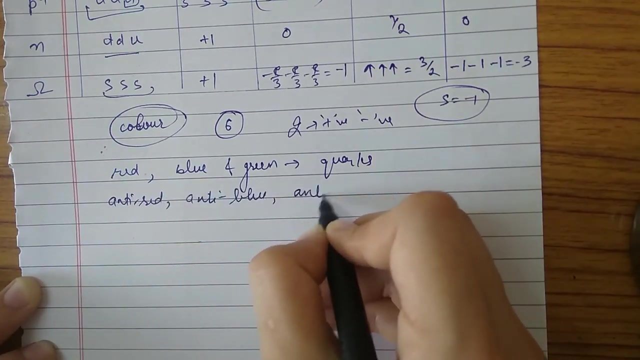 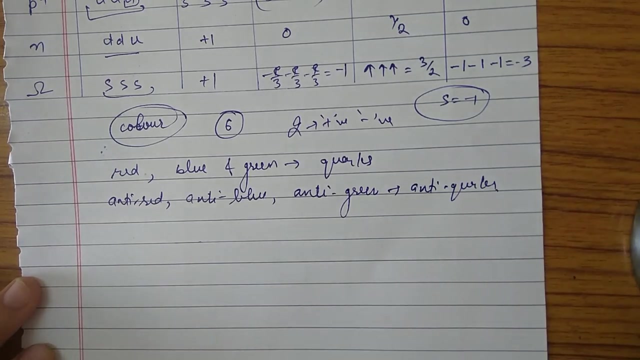 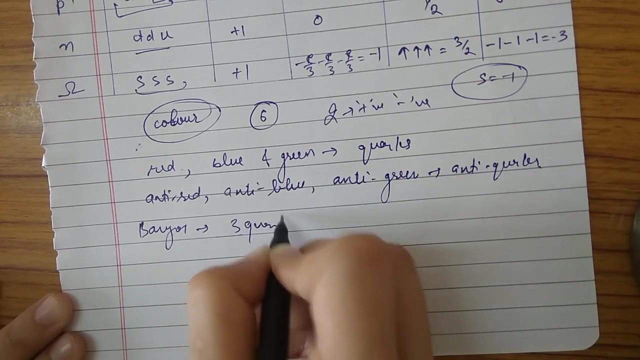 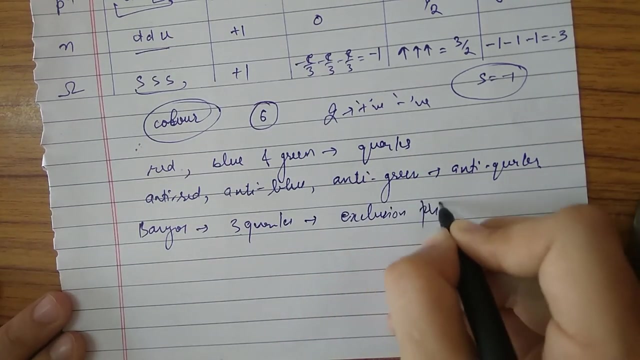 It was assumed that there were red, blue and green color for quarks and anti-red, anti-blue and anti-green for anti-quarks. Now, therefore, we could say that beryon have three quarks, all having different colors. This satisfied the exclusion principle. It was assumed that beryons have three quarks.